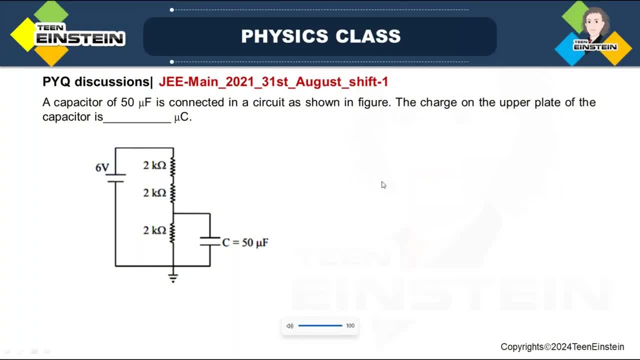 This conference will now be recorded. Very good morning students. Welcome to the PYQ discussions with the physics class. So today we are going to complete the discussions on the paper J. main paper 2021. 31st August. SIPT 1 paper. 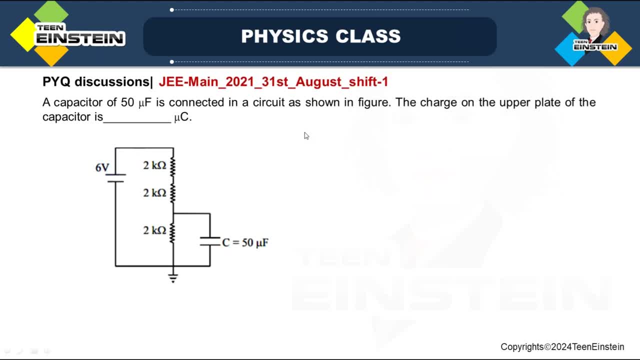 So let us start our discussions. Let me change the color of the ink. So here this person says: a capacitor of 50 micro farad is connected in a circuit shown in figure. This is the figure: The charge of the upper plate. 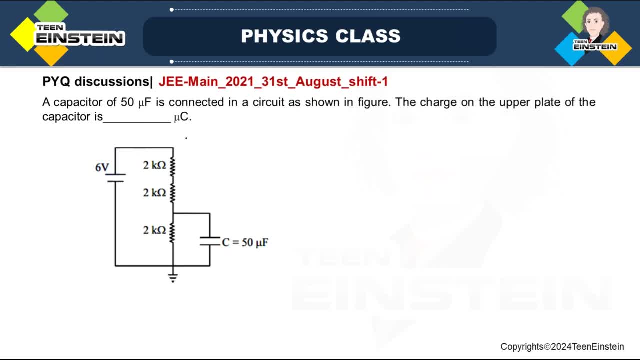 of the capacitor is dash micro coulomb, So you have to find out the charge in this upper plate. In fact, charge will be the same in the upper plate and lower plate as well, but the sign will be different. Okay, 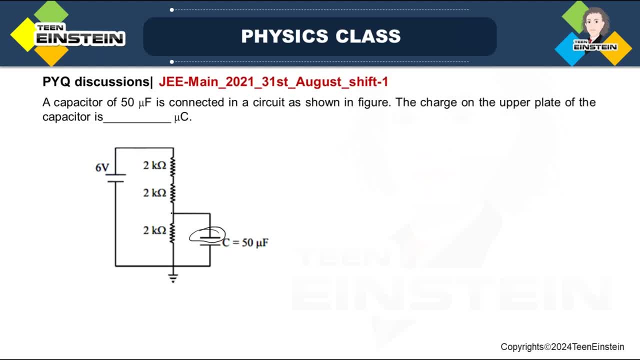 So we know, see, this is a six volt DC battery, So there will be flow of charges through this and this capacitor will get charged and hence it will store some charges. And you look here: this point and this point are same for this register. 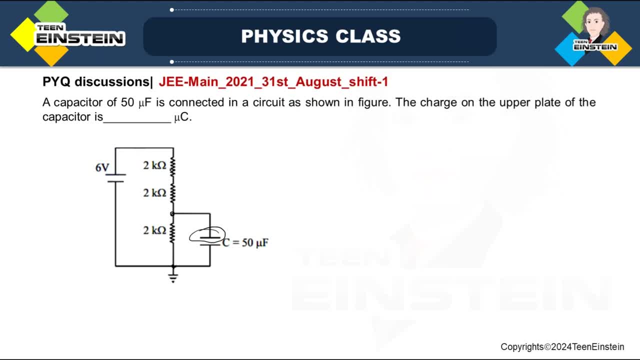 as well as this capacitor, And all three registers are actually identified. And all three registers are actually identified, Identical: Two kilo ohm. two kilo ohm. two kilo ohm. Okay, So the voltage drop across each. 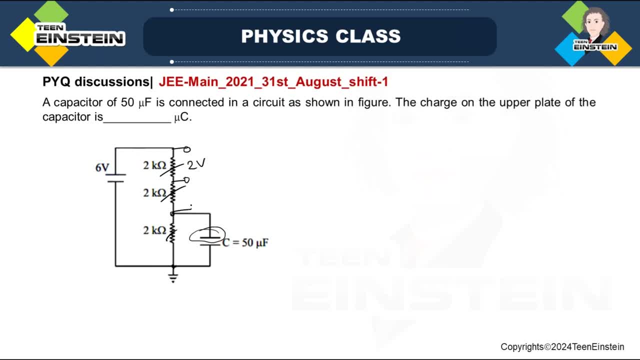 across each will be two volt. Two volt, Okay, And across this also will be two volt, so that it will be total two volt. And since this capacitor is connected across this register, So we'll have this capacitor connected and this capacitor is connected across this register. 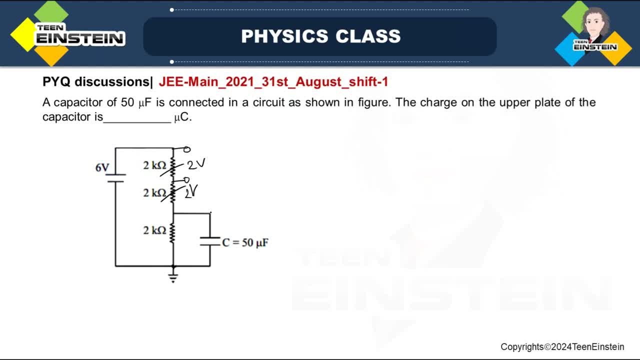 So we will have potential difference across this capacitor also. 2 volt. Okay, so there will be 2 volt, Okay. so when we know the voltage or potential difference across the plates and the capacitance, then what else you require to find out the charge? 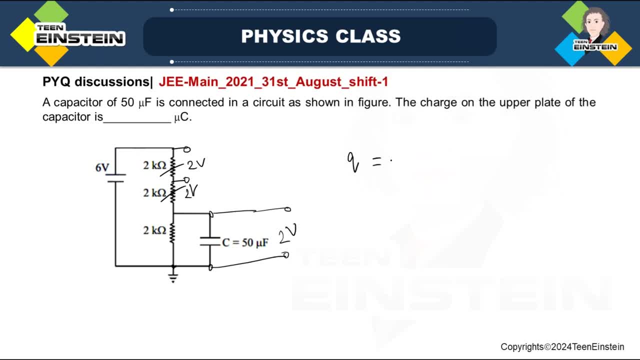 So you know the formula Q is equal to C into V. V is the potential difference across the plates and C is given. So this is micro farad, C is script micro farad and this is in volt. So it will be actually 100 micro coulomb. 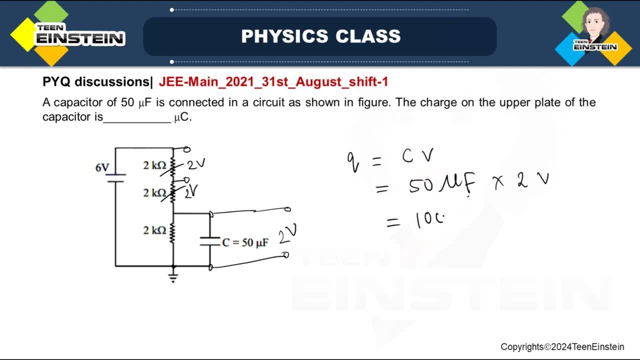 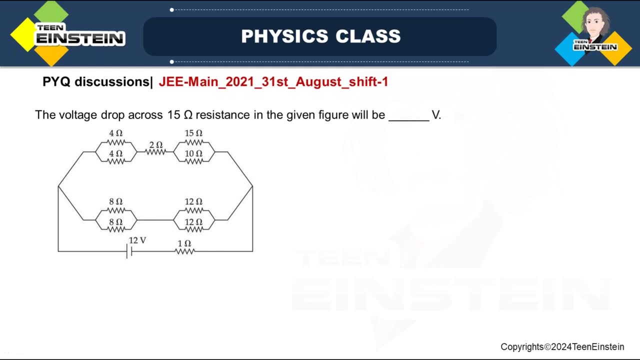 So farad into volt will be coulomb. Okay, so it will be 100 micro coulomb. Okay, so this is 100. Okay, all right, let us go to the next problem. This problem is also very, very simple problem, if you can do it in cool mind. let us see. 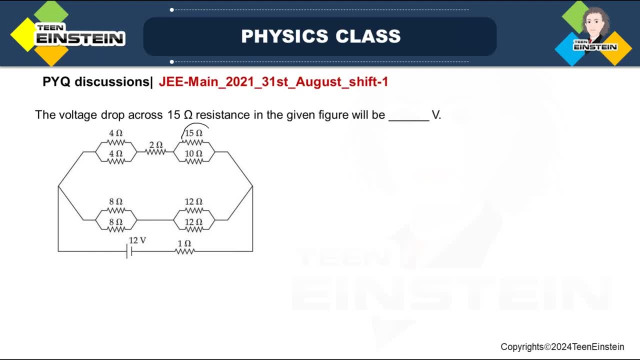 this figure: Okay, we have to find out the voltage drop across this 15 ohm resistor in the given figure. Okay, So here you look, this 12 volt battery. Okay, This battery is connected to this parallel branch, as well as this one ohm resistance. 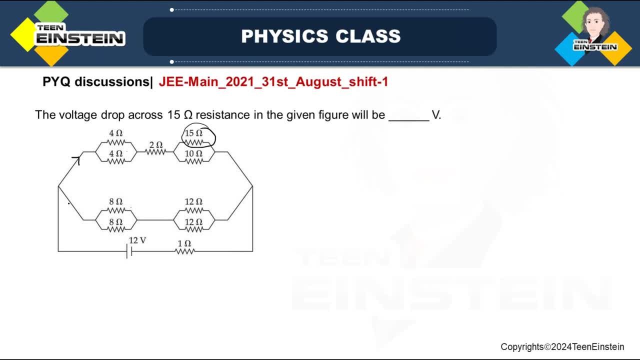 First of all, I have to find out what is the current flowing through these two branches At least. I need to know what is the total current first. Okay, total current. and then I need to know what is I1 flowing through this branch. that will flow through this whole branch itself. 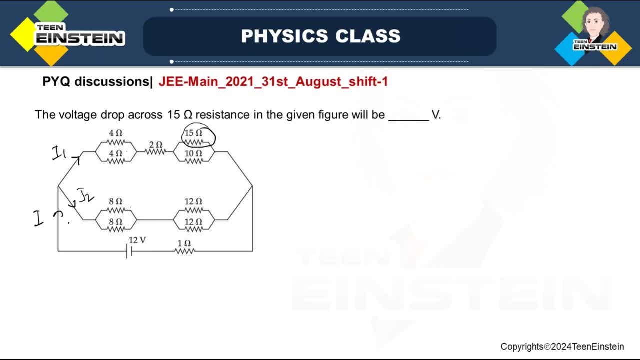 Okay, So I1 and I2.. Okay, these are the two main things we can actually find out. So how do you find out that? So for that better, to find out the equivalent resistance for these two branches. Look, this is actually parallel branch four, four. so four into four, divided by eight. 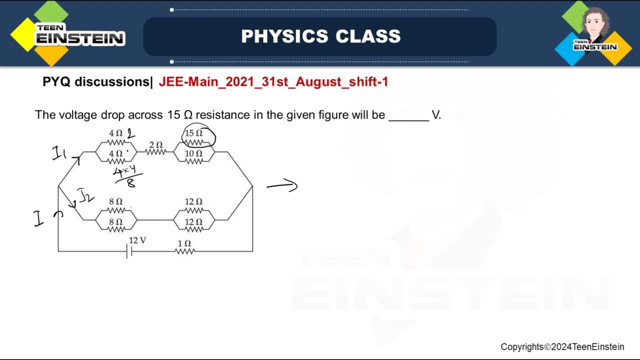 So this will be two. So I have got two out of this two. I have two already here in series And this is 15 into 10 divided by 25.. So this will give you six. So look this that this is two to four and six. i have got 10 ohm resistance in the upper branch. 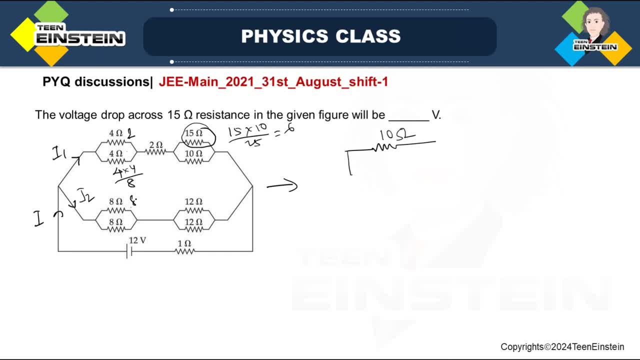 and the lower branch. i'll get here eight into eight, sorry, eight into eight, divided by 16, so this will give you four here, and this will give you, see, 12 into 12, by divided, by divided by 24, so to 12: 2, 6, so this will be actually 6.. so i have got resistance in the both branches as 10 ohm. 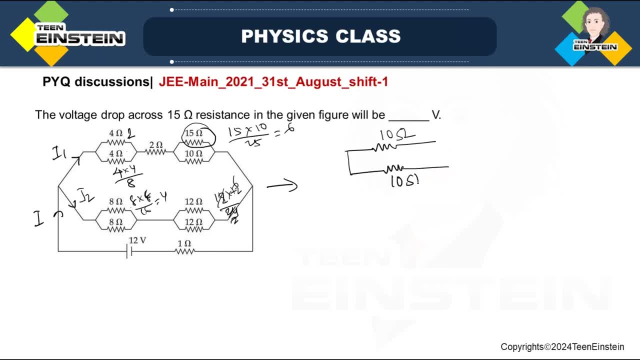 okay, 10 ohm. so here also 10 ohm. and i have got another resistance, one ohm, one of them. so this is connected now with this 12 volt battery. okay, 12 volt battery. now what is the total current? see, this will give you 100 by 20. 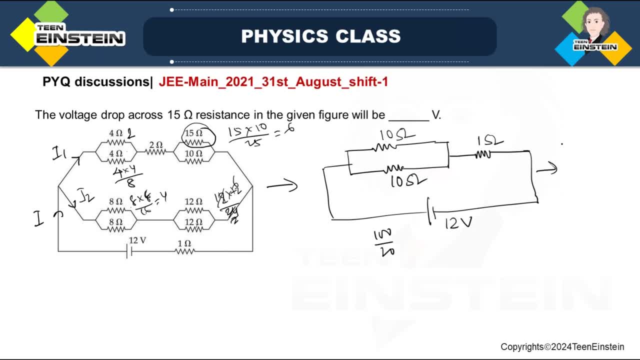 so this will actually equivalent, will be see: equivalent resistance will be then 6 divided by- sorry, 6 ohm, okay, 6 ohm ultimately. so this is 12.. so the total current which is coming out of the battery will be actually 2 volt. sorry, 2 ampere. okay, so the total current coming out is 2 ampere. 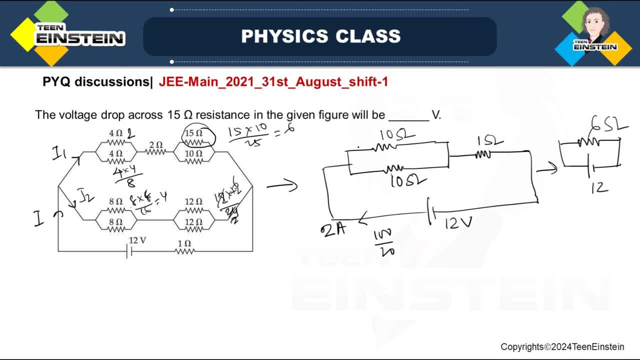 and since these two branches will have the same equivalent resistance, so through this there will be: i1 will be 1 ampere and i2 will also be 1 ampere. so there is no decal. you can see there is no, you have the volume value and it will take. 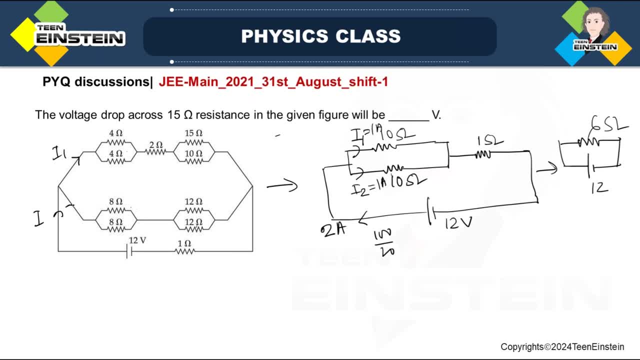 away the power supply. so this is 111ohm and it will call the power supply output to 21.. 21 ohm. okay, so it will take away to expected value i1 ohm. 22.3 vam –0.214…. 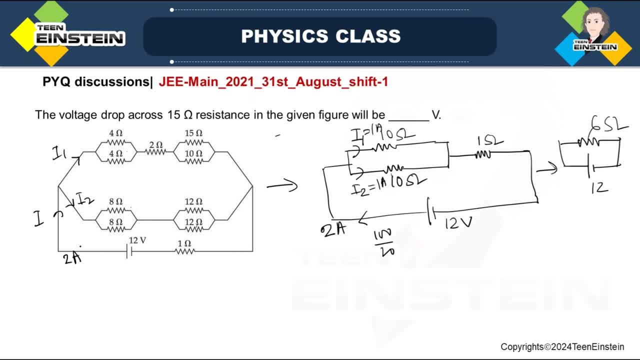 this total current is two ampere which is flowing through or coming out from the battery. and, okay, so this is one ampere. this is also one ampere. so this much i know. now, see, i have to find out. see up to here, there will be one ampere current coming up. okay, one, i one. 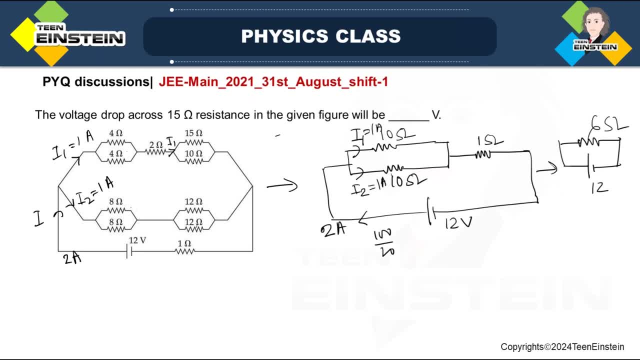 then this will be again branched through these two parts. okay, so i have to use here current division. okay, formula for the current division of current. i have to find out current through current through 15 ohm. so what? i have to write the total current, that is the 1 ampere or i1 here, into the resistance. 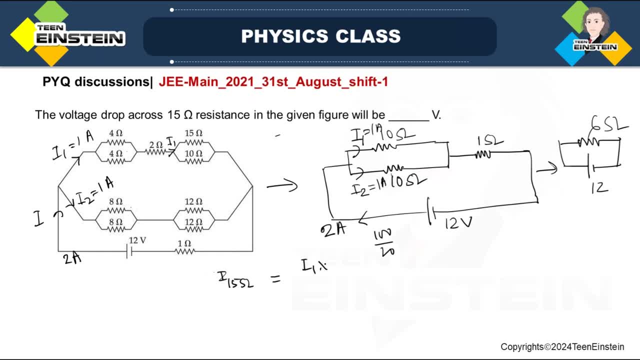 which i'm considering. that one i should not write. i should write the other resistance, that is 10 divided by the total resistance, that is 10 plus 15. okay, so this will give you the current through the current, through 15 ampere. this is actually current division formula. okay, division of current. 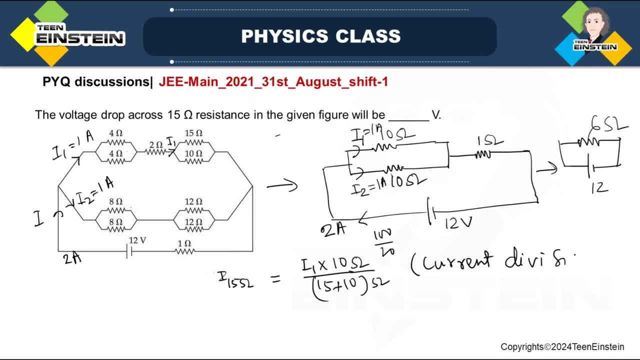 current division. this is actually the current of the voltage in the reading of the current. so it is positive. because of this resistance, because of this resistance, i am not able to do that- these two will actually have same voltage. that i'm not able to do here. obviously this two will have same voltage. that is fine. but i cannot success further with this. better, to find out the current, you have to find the current of current division. 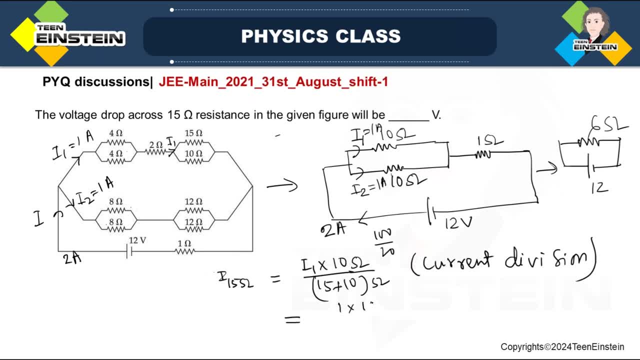 so this will be see. this is 1 ampere divided by see. 1 into 10, divided by 25, which is actually 2 by 5, which is 0.4. okay, so 0.4 ampere i have got. now i have to find out what is the voltage. 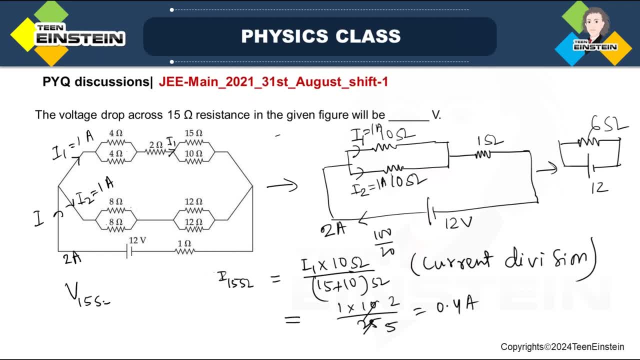 across this 15 volt. okay, sorry, 15 ohm. so current into volt, sorry, current into resistance ir. so what is the current flowing through this? 15 ohm? that is 0.4, sorry, 0.4 ampere into the resistance, that is 15. so this will be actually 6 volt. 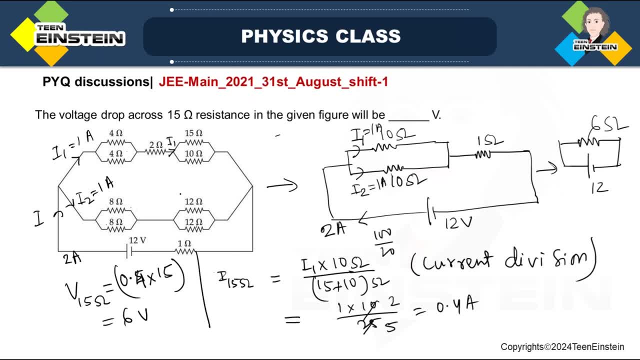 okay. so what is the voltage? 6 volt, okay, and this will be the answer for this question, actually, okay, so 6 volt will be the answer. so 6 volt is right. 6 volt will be the voltage drop across 15 ohm resistance. okay, so this is all for this. 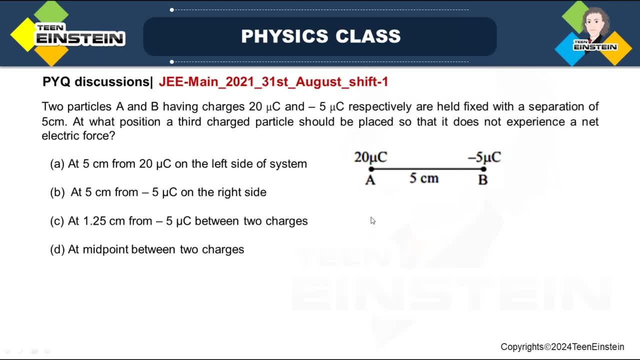 you, you question. let us go to the next problem question. let us go to the next problem question. let us go to the next problem. okay, this problem is also very, very okay. this problem is also very, very okay. this problem is also very, very simple problem, simple problem. 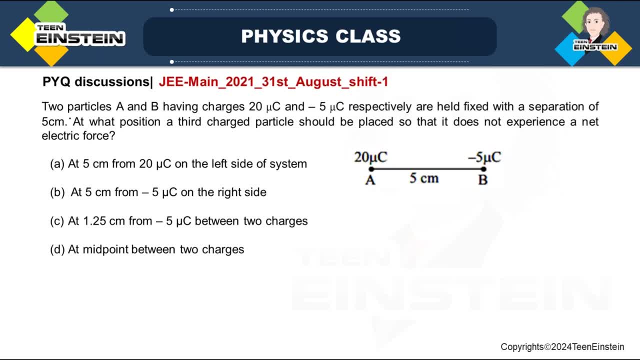 simple problem: this is from electrostatics. let us: this is from electrostatics, let us: this is from electrostatics. let us see this problem. see this problem. see this problem: two particles, two particles, two particles. particles charge particles a and b. particles charge particles a and b. 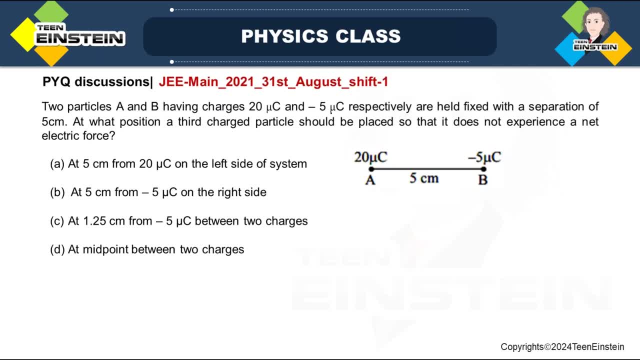 particles charge. particles a and b: having charges: having charges: having charges: 20 microcoulomb and minus 20 microcoulomb and minus 20 microcoulomb and minus 5 microcoulomb, 5 microcoulomb, 5 microcoulomb respectively are: 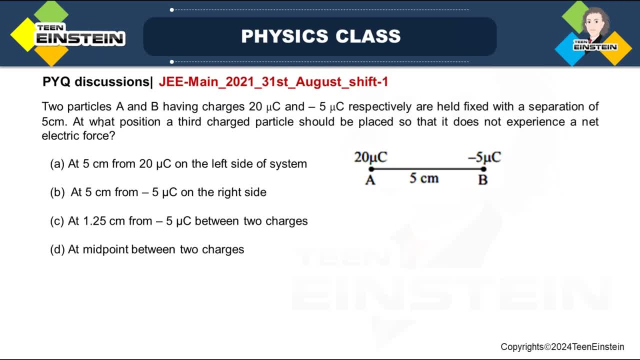 respectively are respectively: are held fixed, held fixed, held fixed with the separation, with the separation of five centimeter. at what position a third charge charged particle should be placed so that it does not experience innate force. so i have got two charges: 20 microcouple and minus. 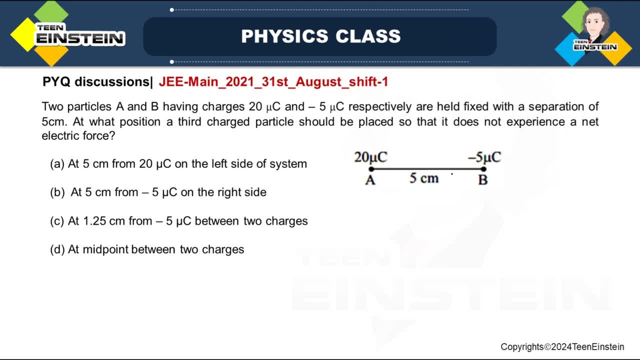 two minus five microcouple. they're separated by five centimeter, so i have to get a third charge. let us say that charge has like that, that charges small q, so i have to place this charge at a place such that such that there will be no. 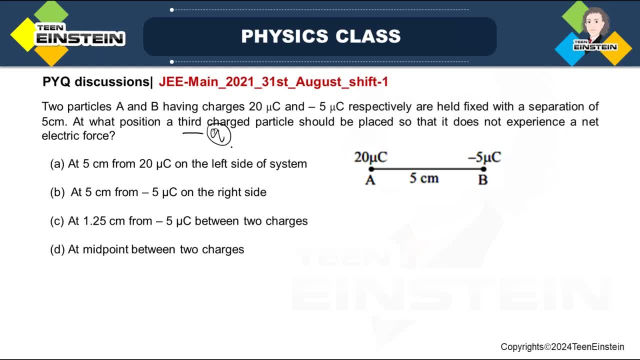 need force experienced by this charge. okay, that means you know, if i keep a charge, let us suppose we are placing the charge on the axis of these two charges itself. okay, in the same line, but where to put the charge, whether i should put the charge here near to 20 micro Coulomb or near to minus five micro Coulomb. So which one is logical? 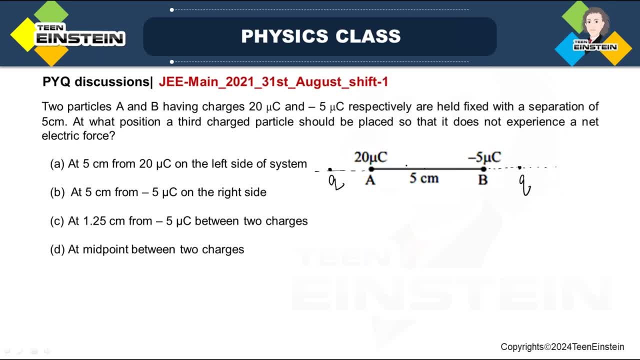 or I should put in between here somewhere. See, logically, this has got more charges. See, much more. this is minus five, this is actually 20.. So this has got very, very large charge. So to balance the force given by this 20 micro Coulomb charge on this I have to. 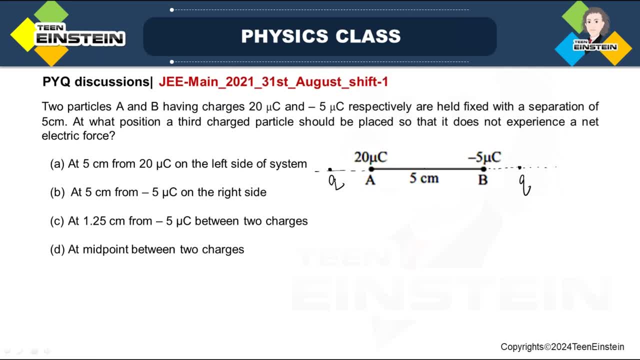 somehow keep this charge in a way that this force, like the force applied by this minus five micro Coulomb, at least becomes equal. Okay, It becomes equal at least. So for that, you know, if I just keep me at this, see at this particular position, or left to the left. 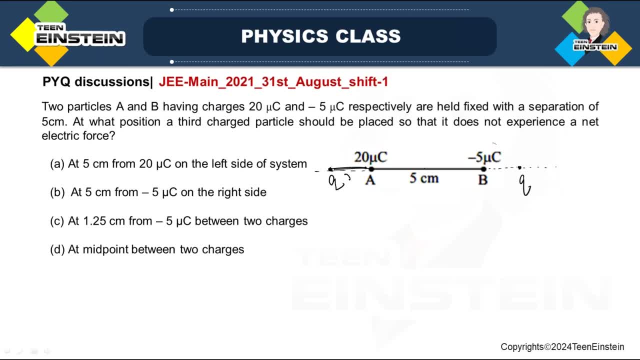 side to the 20 micro Coulomb, then this is actually nearby. This is supposed. this distance is less than this distance, you look here. So the charge is also less and the distance is also very, very small. So you know, the Coulomb force will be one by R square. right It varies one by R square. 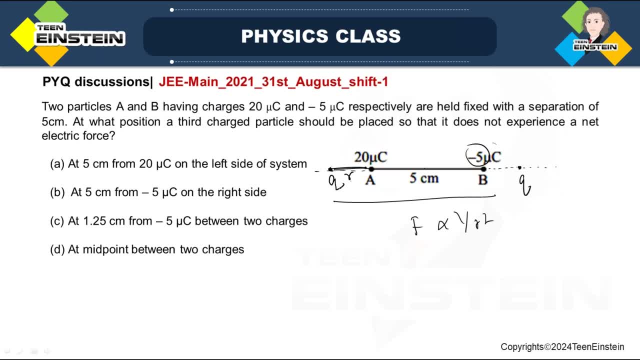 So the force applied on this Q charge- third charge- by minus five micro Coulomb- will be really very, very less than the force experienced by this Q charge due to 20 micro Coulomb. So the logical point will be: keep the charge. Now I will do the same thing again. So let us say I have five micro Coulomb. 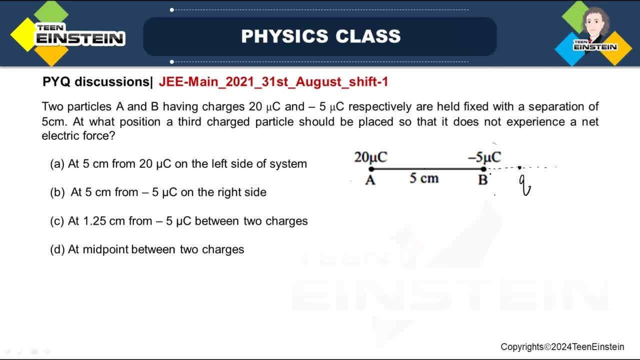 Let me, let me just find the distance. that means I have negative zero. So now let us take the distance of positive zero. I've taken negative zero, negative zero, So I'm taking the distance negative by negative zero. So the force applied by this Partan charge is negative zero. that means minus five micro. 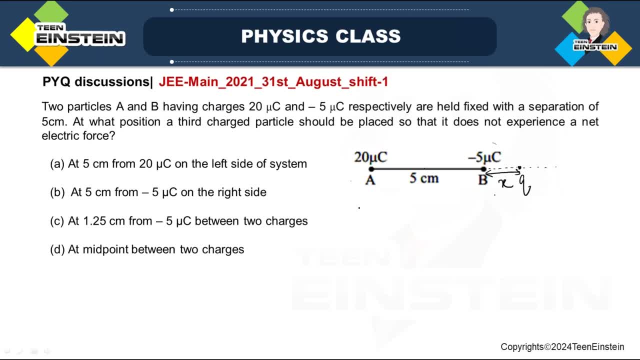 Coulomb charge. Okay, Okay, Okay, Okay. Okay. the problem: these two forces, the force applied by 20 microcoulomb will be exactly equal to the force applied by minus 5 microcoulomb. okay, on this q chart, so i can write k, q into. 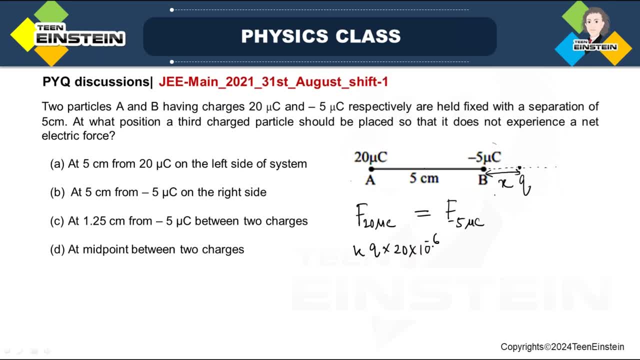 20 microcoulomb divided by r square means it is: it is actually 5 plus this. like 5 plus x whole square, this will be exactly equal to the 5, the force. i am taking the magnitude 5 q into 10, to the power minus 6. 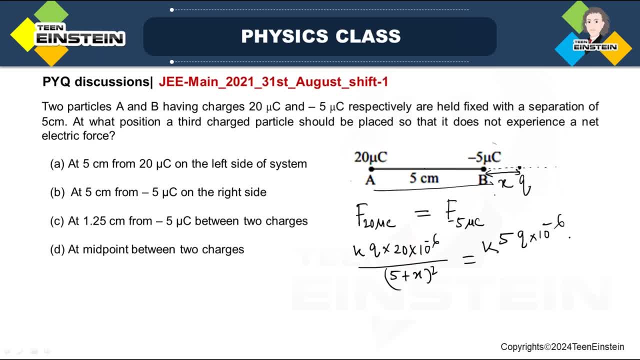 k will be here. so k, q, q divided by r square, r square is actually x square. now look these two things here: this q, this q, i can strike out. this k are constant. this 10 to the minus 6, i can strike out. so what i get? see, i get 5. i can actually simplify a little bit. so 4, see, i get 4 x square. 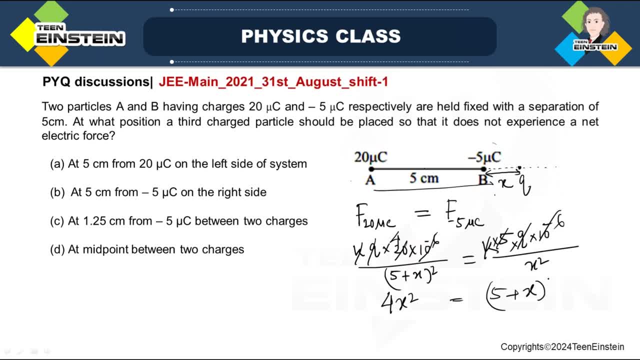 is equal to 5 plus x, whole square right. so from both side, if i just take square root, i get 2x. i'm just taking the positive plus or minus. it should be, but i'm taking this positive plus, so this is 5 plus 2. now this will give you. x is equal to 5 and this is in centimeter. okay. 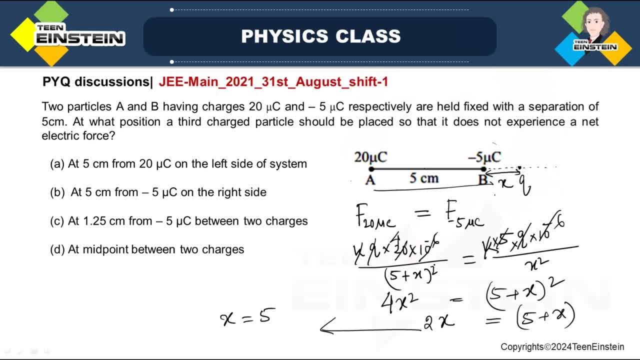 turning positive and this is in centimeter. all right here. actually i should have written 10 to the power minus. okay, centimeter, let it be both side anyway. you need will go away, okay the answer. so x will be actually five centimeter, five centimeter, and that is actually right side. 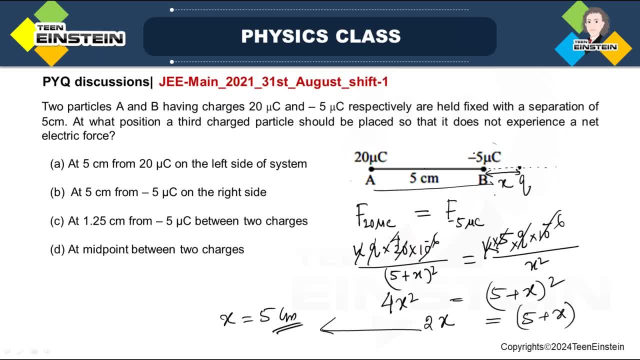 of the charge minus five microcoulomb. let us see the options. at five centimeter from 20 microcoulomb on the left side of the system. no, this is wrong. at five centimeter from minus micro, minus five microcoulomb on the right side. it is actually true. others will be obviously. 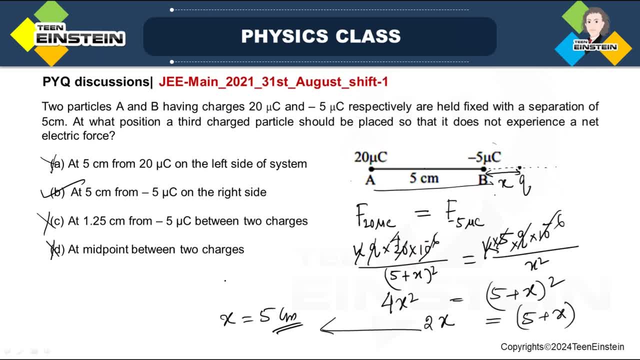 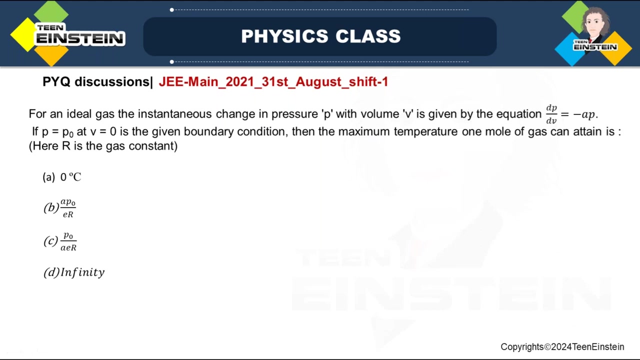 not true. okay, so we have got b to be the correct answer for this question. okay, oh, i'm sorry. uh, this is yes. yes, yes, this is fine. yeah, okay, so the right side: yes, this is the answer. okay, now we have got another problem. this is for an ideal gas: the instantaneous change in pressure. 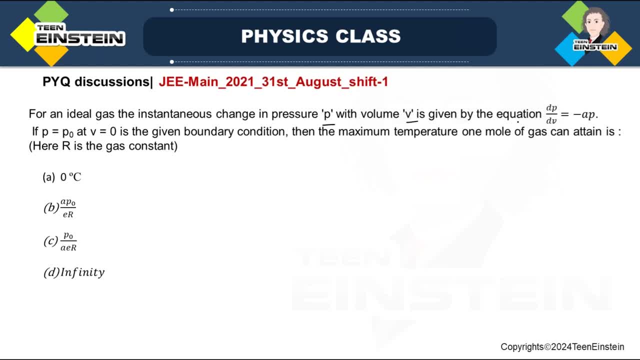 p is with volume. V is given by this equation: dP by dV is equal to minus AP. so a you have to take as a constant over here and P is the pressure, instantaneous pressure. so the question is saying that if this instantaneous pressure is P 0, 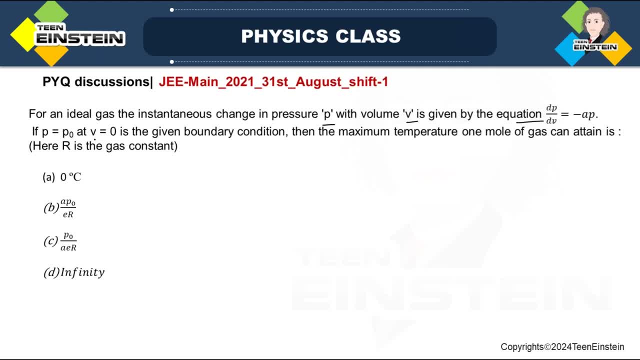 some time. then you know this will be. volume will be 0. that means this is the boundary condition at V is equal to 0. that means where the volume is 0, the instantaneous pressure will be P 0. the maximum temperature of one mole gas can attain is how much out of out of this four options see: 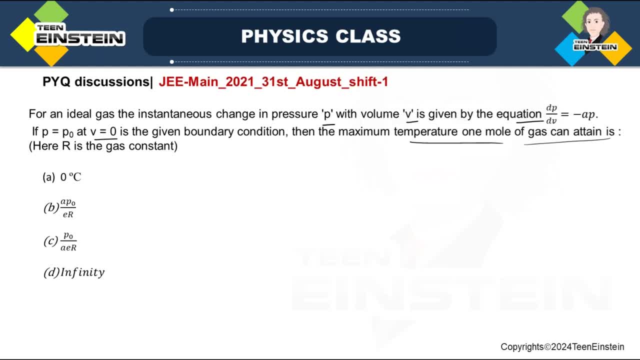 so we have to find out the temperature, maximum temperature attained by this process. okay, so we have been given dP by dV is equal to minus AP. right, let us do the integration. so I'll keep this dP by P here and minus a. sorry, a dV. okay, a dP. 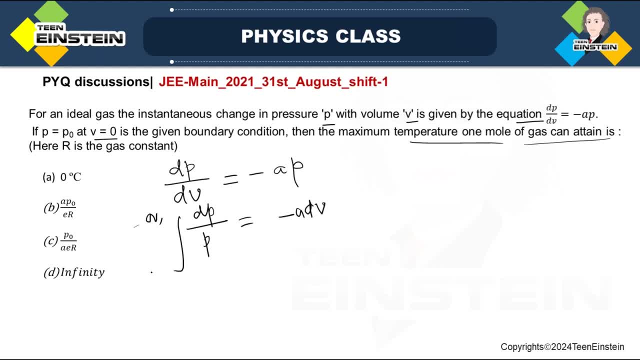 now integrate it within the limit. see, when V is equal to 0, V is equal to 0, then P is equal to P 0. okay, this is a the boundary condition, and let us say, the final volume is V, when this will be P. okay, so this will give you see, ln. 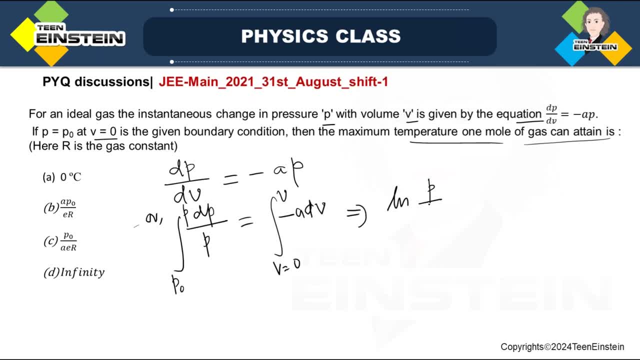 this integration. if you do, you will get ln P by P 0. okay, this P is upper limit, this is lower limit, and on the right hand side you will get a into V. this is the thing you get. okay, now see, from here actually you can write: P is equal to P 0, e to the power minus a V. 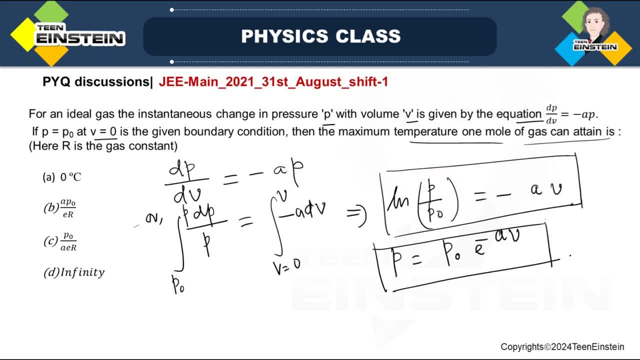 this I can write. you can just check it: P is the instantaneous pressure and P 0 is the pressure when the volume is 0. now I have got the expression for the instantaneous pressure right. can you write: PV is equal to RT for one small gas. yes, I can write this. so from here, see if I put the value of P over here. 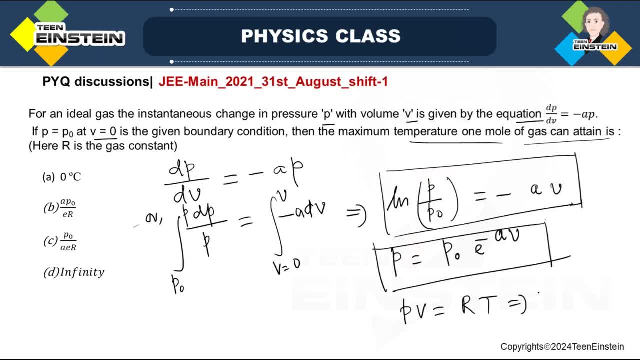 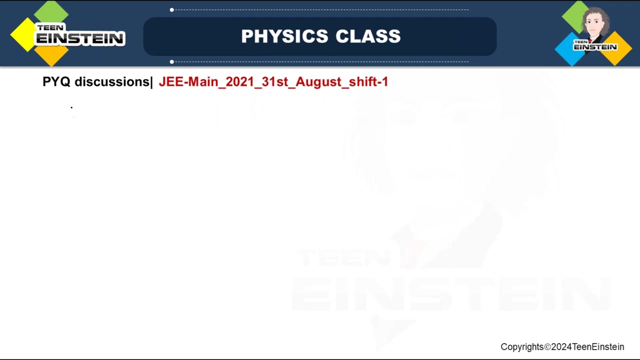 okay, so what? we will get so P 0. I write P 0 e to the power. okay, I have to find out T actually. all right, just a minute, I just go to the next page. so I have got this expression. let us go ahead with this, so we know. PV. 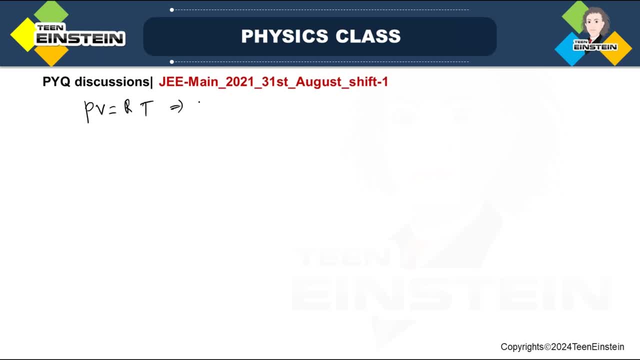 is equal to RT for one mole gas. so from here I can write: temperature: T is equal to PV by R. so what is P? we have got P 0, it is B. is there e to the power minus a? this B is- I'll write similar, some kind of rotation- okay, so this is B divided by R. okay, this is fine. okay, now I. 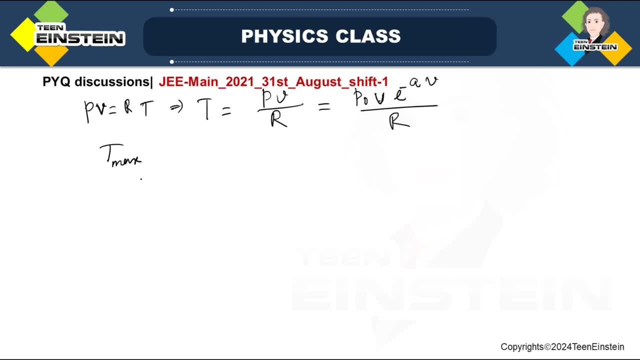 have 200. what is T max? so for T max, I can write, you can write, I can write this: P 0, but that will be V 0. so I do not know how I dt by dv equal to zero. now let us find out the values of v. okay, values of v, or sorry, i have to find out this. 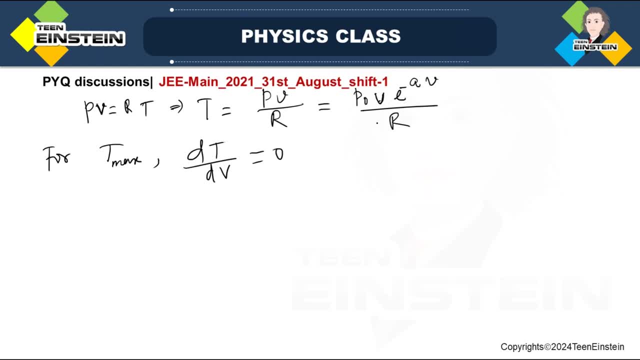 uh, a i have to find out the value of a for which i am actually going to get maximum temperature. what is the value of this a when i am getting maximum temperature? okay, so let us put this: dt by dv is equal to zero, so this expression we know. 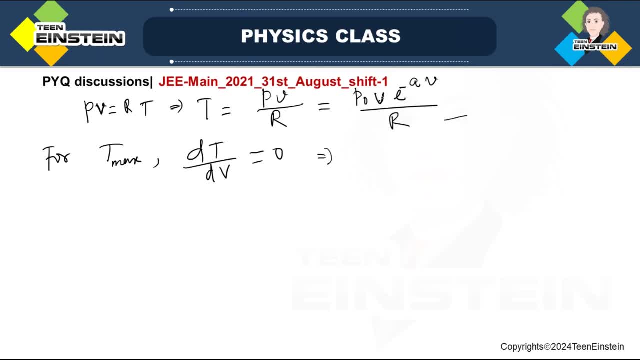 so dt by dv. this is actually say, if i just take derivative with respect to v. so first term it is by minus a v by r, minus a p, 0 v by r. into the part minus a v, this i have to put zero. so look then. 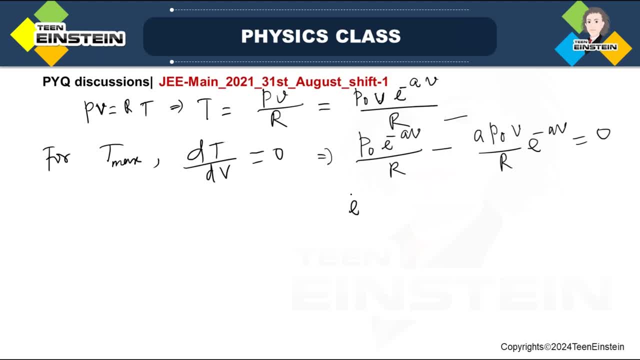 we get see it is the power a v. okay, it is about a v if i take common, so this one, this one, actually get cancelled from both side if i take them say this actually: okay, let us just keep this b zero and all okay. it will give you better understanding. 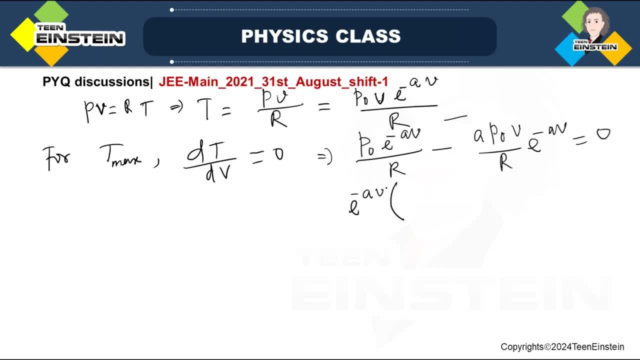 so let us take a v 0 common. this one, it is the power minus a v common. so i have got p 0 by r minus a v p 0 by r. this is equal to 0. so either this will be 0 or this will be. 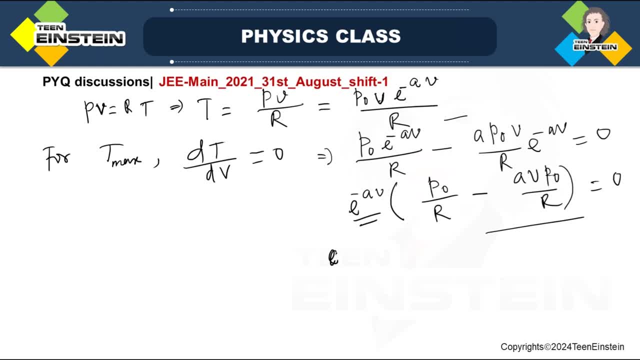 0.. so if i put this is equal to 0, then you know this: a v has to be infinity minus infinity means 0. so i get actually: a is equal to a is equal to infinity, right from there, sorry, infinity, so infinity i should not take. 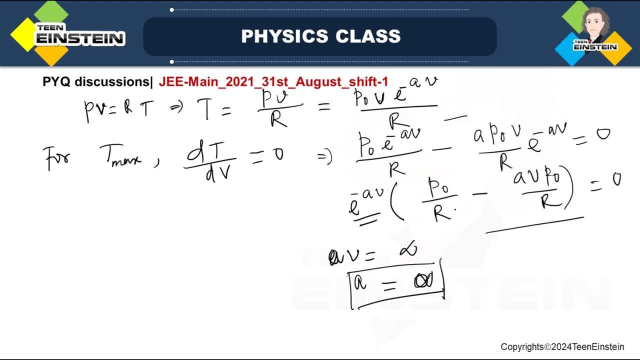 so i should have another values. let me see from here. okay, so if i put this term 0, then i get cp 0 by r, a v 0 by r. so this term will cancel each other. so a will be 1 over p. so i get a is equal to 1 over v. 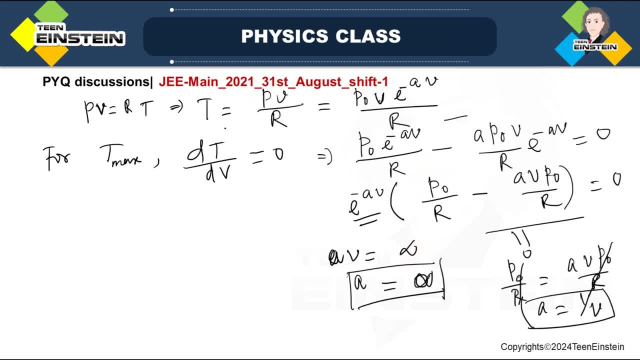 so i'll put the value of that a in this expression, in the temperature expression. so expression for the temperature we had got, t is equal to p, 0 v e to the power a v divided by r. okay, so t max will be what will be t max. for t max i have to put the value of. 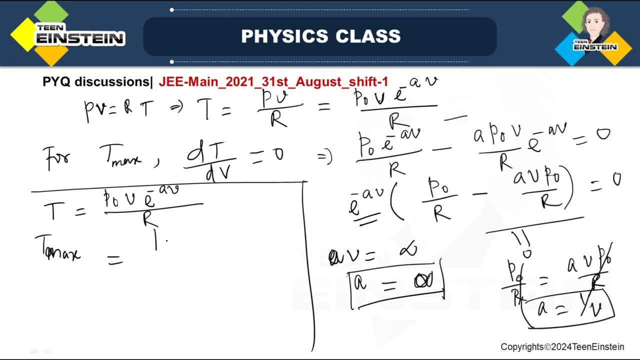 a, a. i have got one of one over v, so p 0 v e to the power minus 1 over v. a is equal to 1 over v means e to the power minus 1 divided by r. okay, i think somewhere i have left one a. 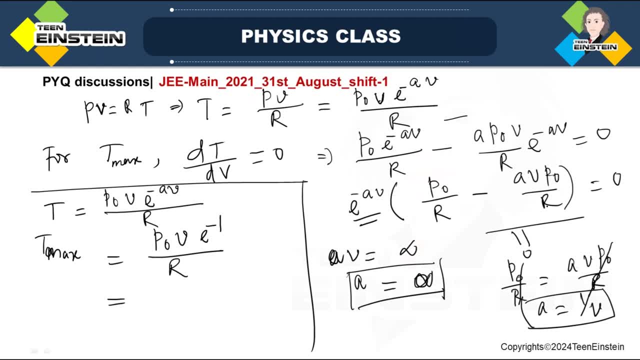 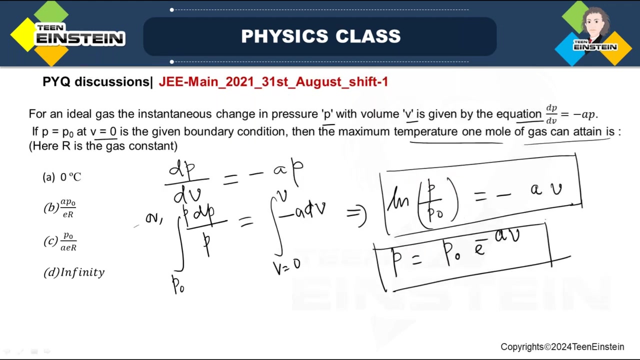 i have a over here. okay, fine, a, yes, fine. so what is the value of temperature? sorry, uh, what is the value of this? okay, so p, v, 0, v e r. okay, look the options. okay, we have in terms of a instead of v, let us put the value of v anyway. these are. 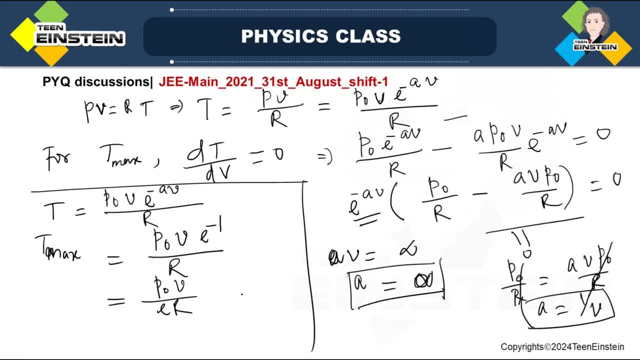 this will be e to the power minus, so v will be actually one over a right. so i have the values in terms of one over. okay, so in terms of a. so i have to put the value of a, so v is equal to. i'm sorry, uh, we have to put the value of v in terms of a. 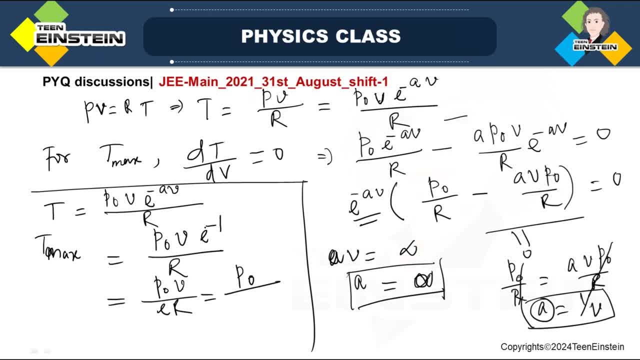 v is equal to. if i would have put here, let me just put there itself, okay, this is say i'll put the value of v. v means 1 over a, so this is 1 over a, and this will be e to the power minus 1 only. so this, this is going to be a e r, okay. so what is the value of this? t max? t max is: 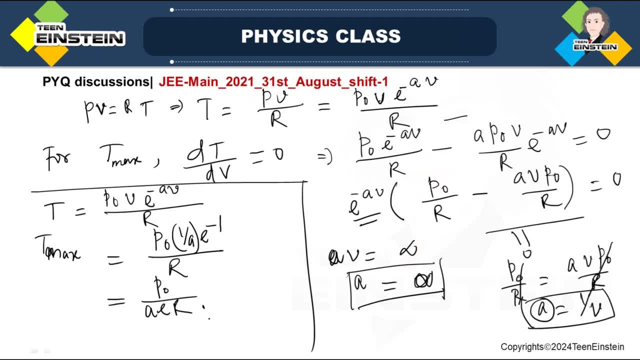 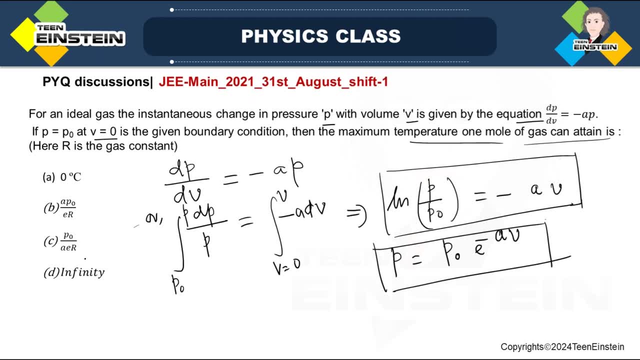 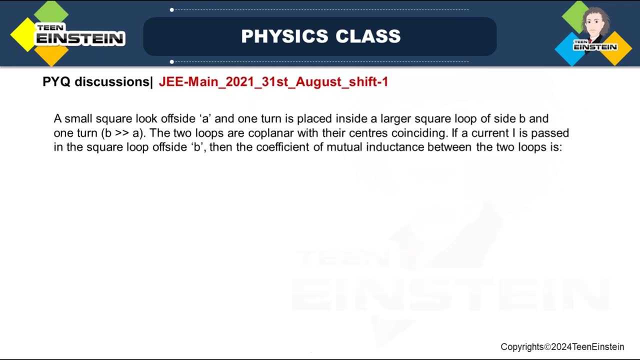 equal to p 0 by a e r. so this is actually the answer. let us see: t max is equal to p 0 by a e r, so option c will be the correct answer for this question. okay, so let us go to the next problem. this is really a very good problem. let me give you the 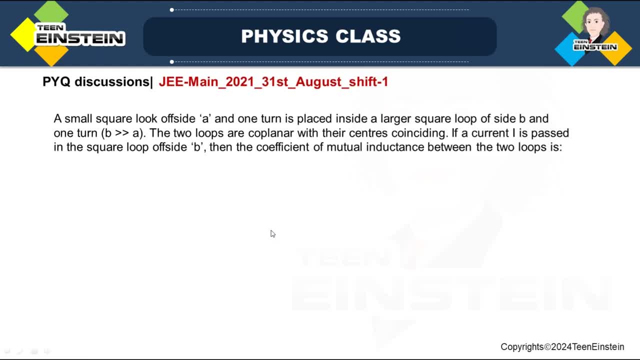 options for this question. first let me read the question and then give you the options for this question. okay, so the question says: a small square, look upside, square, look upside. that's a option. this is actually. this is off side a a square. this is loop, actually not look a square loop. okay, a square low. 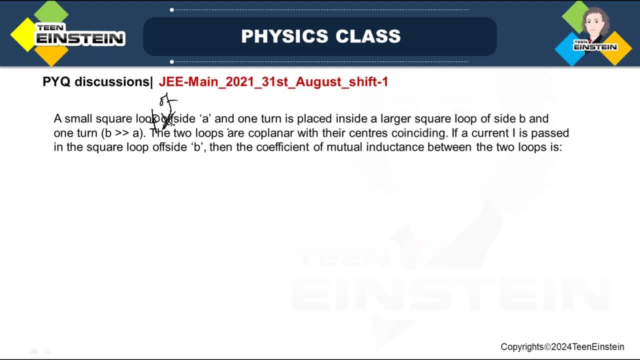 a small square loop of side a and one turn is placed inside a large square loop of side b and one turn 2, 1, 2, 2, 3, where b is much, much greater than a. that means you know you have a big square. look like this. okay, i don't think this is perfect square. let me just 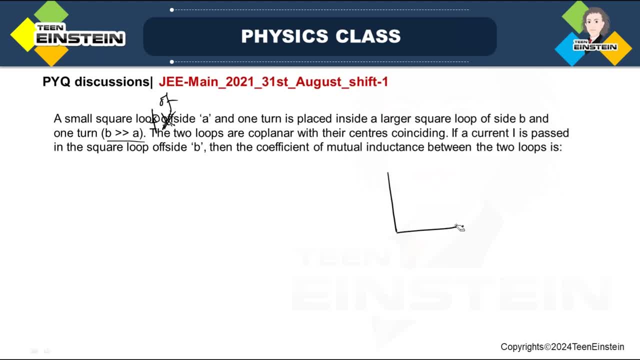 redraw this. this has got greater length. okay, so this is somewhat square. okay, this is a bigger, bigger square loop which is side b and inside that there is a smaller square loop, and see, the two loops are co-planner, with their centers coinciding. so if i say this is the center, so i have got another square loop over, 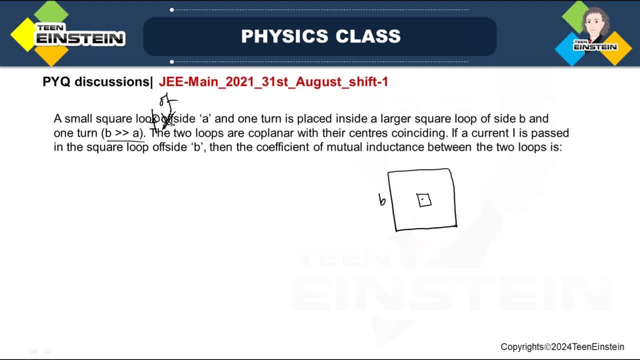 here. okay, another square. look like this. so this is the center. so this is the center. okay, so which has got? let me redraw this, sorry. okay, this is the small loop. okay, so the centers are actually coinciding. now, if current i is passed in the square loop, b suppose current i is passing. 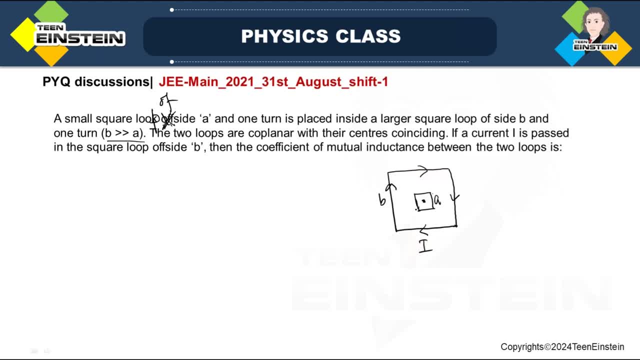 through this square loop b off-side b- this is not off-side, this is off-side b. then the coefficient of b is not a step coefficient of mutual inductance between the two loops. then coefficient of mutual inductance between two loops will be see. there are options given over here. 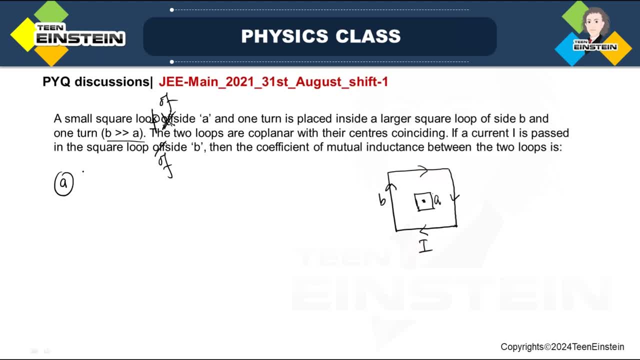 let me write down the options. first option says it is mu 0 by 4 pi b and in the numerator it is 8 root over 2. ok, option b says mu 0 by 4 pi into 8 root over 2 b square. 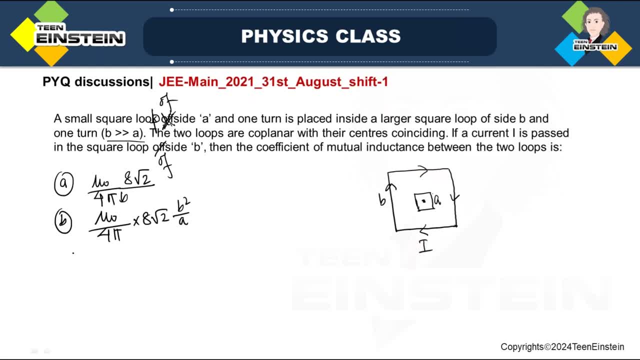 by a ok. option c is 8 root over 2: mu 0 by 4 pi a 8 root over 2. and option d is mu 0 by 4 pi 8 root over ok. this is b: 8 root over 2. 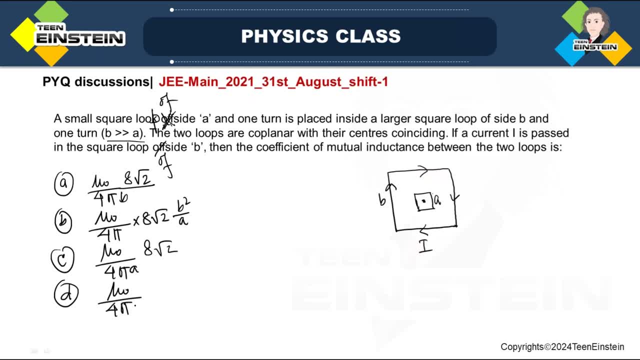 and option d is mu 0 by 4, pi 8 root over 2 and the number is mu 1 and number is b. so let us write this as a l by big. ok, so these are the options. you have to find out which one is the correct. 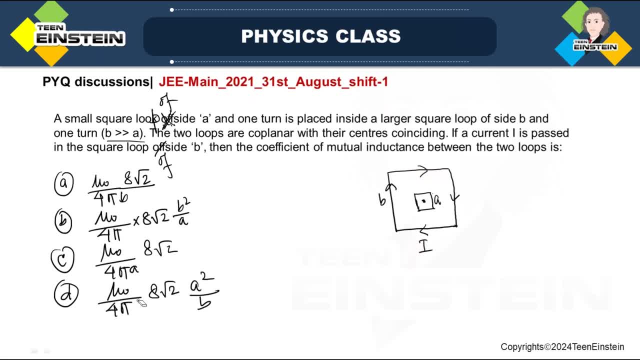 ok, so whenever we go for calculation of mutual inductance or self inductance, whatever you say, let me clean this. ok, it is looking bad, but if we go to the next part and we are going to see that the natural inductance of the input is not correct, which is not correct, which is correct if we are saying that, it is not correct if this is in the same class as we're not using a formula. 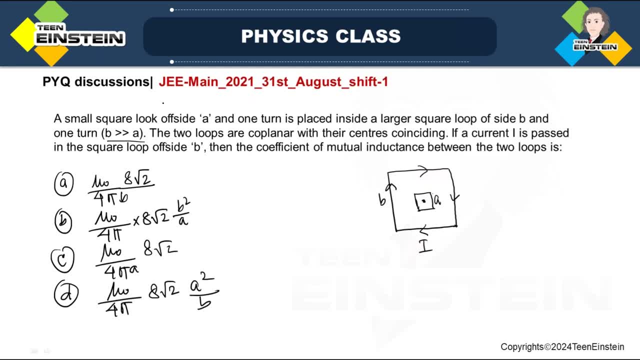 but anyway, this will be off, this will be off, this will be low, okay. so whenever we want to find out self part, mensual inductance, we should actually find out what is the flux, and flux is actually a my mutual inductance or, in case of self, 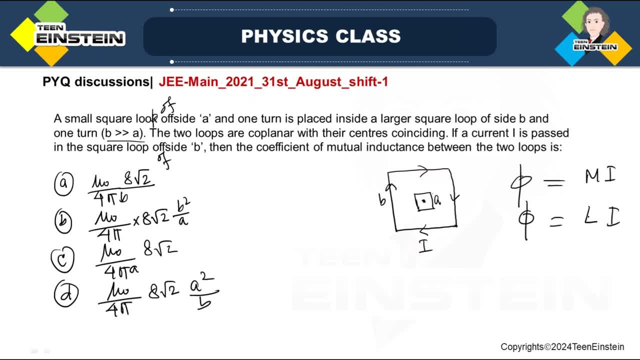 inductance is. it is flux, is equal to phi, is equal to li. so if i find out the flux, magnetic flux, then i have to just multiply with i, sorry, divide with i, so that we get the mutual inductance. rest of the things are easy, right? so how to find out phi? phi is nothing but b into a. 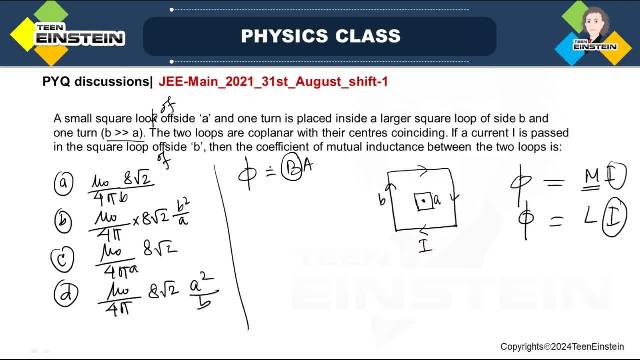 so what is the main problem here? the main problem is to find out what is the magnetic field produced at this center, let us see, and at the center of this square loop? okay, at the center. and what is this area? area of the smaller loop, okay. so, magnetic field produced by the bigger loop at the center, and this is the area a is the area of. 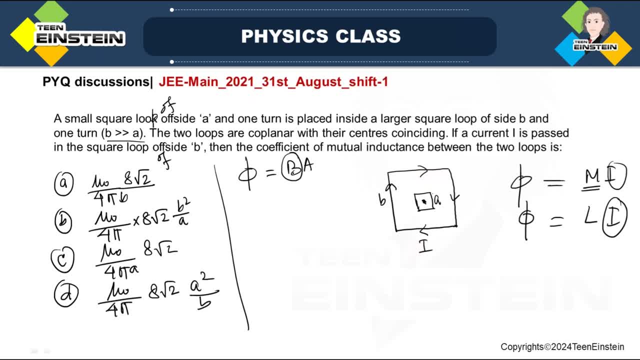 the smaller loop that will give you the flux linked with the smaller loop, and that is is equal to m into i. from there, i will be able to find out what is the mutual coefficient of mutual inductance. okay, let us do that. so what is the formula for finding out magnetic field? 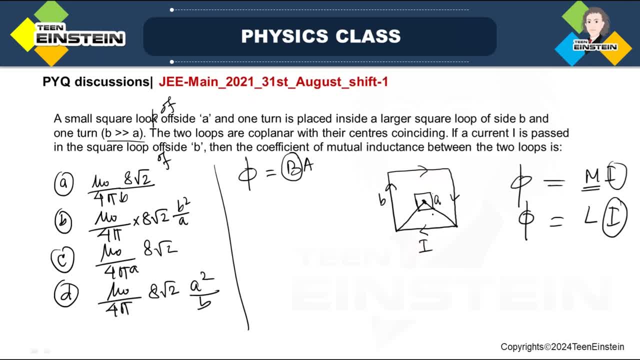 for a finite wire and this kind of problem you might have done n times. okay, you have been given a square loop. okay, of some side a there will be current flowing through the uh, through the wire of the square loop. then you have to find out magnetic field at the center of. 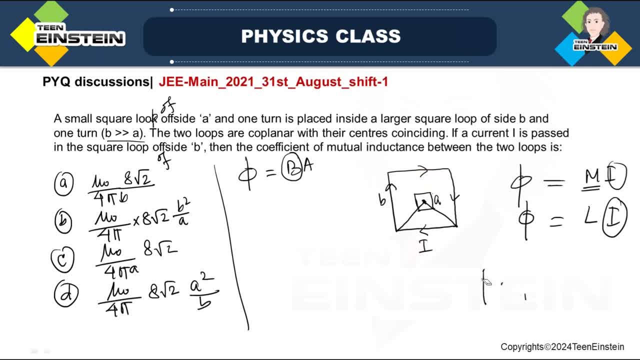 the square loop, so that you know very well, right? so you have to apply the formula for magnetic field produced by if a current carrying wire of finite length, and that you know very well what is that that is actually means. zero by two, zero i by four, pi a if the a is the. 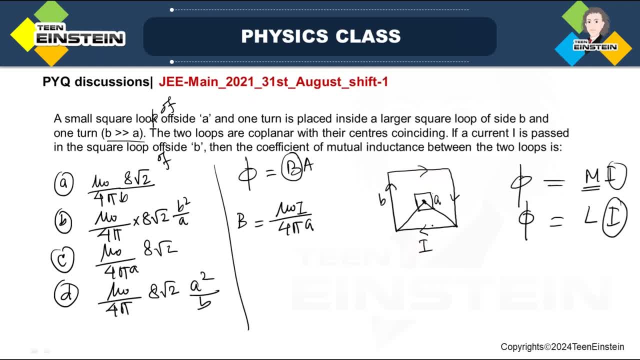 distance from the wire to that particular position, and this will be sine theta one plus sine theta two. okay, this, i know this is the formula. okay for this, how i will apply here. let us see this. so this point is actually see this length. so i have to find out the magnetic field for this. 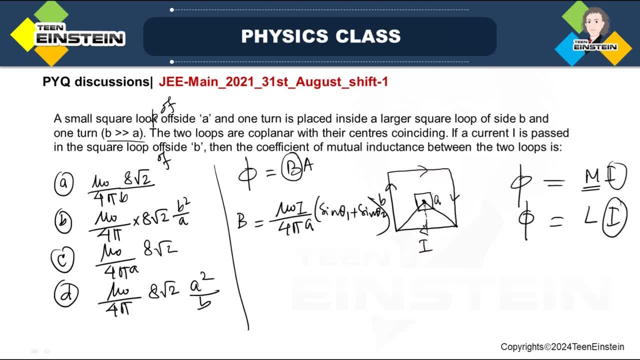 particular where suppose we are taking this particular point? okay, this particular uh side. okay, so see, this is perpendicular bisector of this angle. okay, this one. so this will give you the distance from wire to the point. so this distance is actually b by two, since this is the middle point of the biggest square. okay, and see, this is. 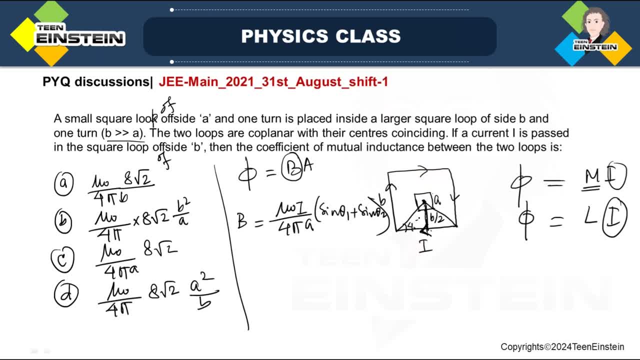 also perpendicular bisector. this is 45 degree and this also will be 45 degrees, since this is 90 degree. okay, so i have got here: this is theta one and this is theta two. okay, so i have got theta one and theta two, so both are 45 degree. theta one, equal to theta two, is that is 45 degree. so this: 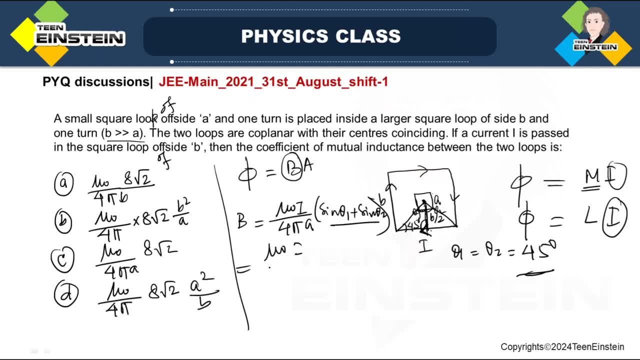 part, i know. then so means zero: i by four, pi, four, pi. what is the distance? this is b by two. okay, right down here now. this is actually both, as theta one and theta two are both same, and that is 45. so this is now two into sine 45 degree. okay, so this is the magnetic field produced. 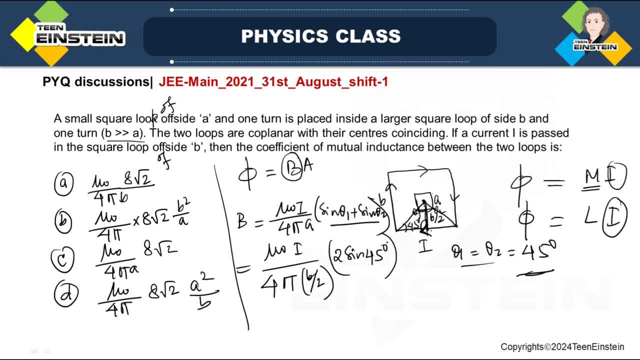 by the single side at the center. okay, now i have to find out the total magnetic field, and that will be four into this b. then what i get, this is one over root two, so let us write that. so means zero, i by four, pi b, and here is two that i'll write here. two. 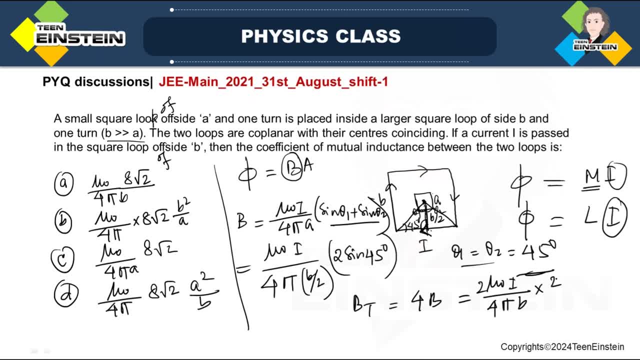 and see this is also two and this 45 minutes, one over root two. right, so better to go with this root two rather than keeping in the denominator. okay, then we have see in the options: i have four pi, so i'm not just striking out this: uh, two million zero and all, so this four pi, let us skip, like this. okay, so we have got. 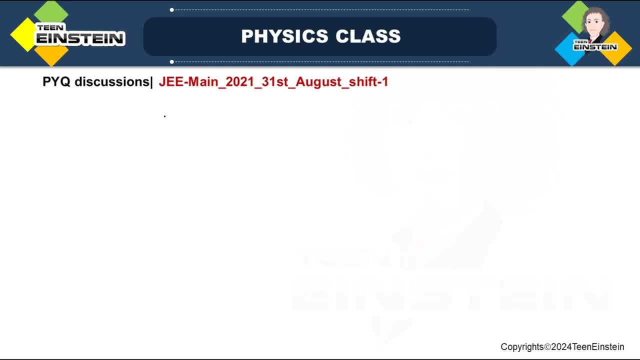 the magnetic field cb total. we have got. what is that? that is two root. two means zero, i divided by four pi b. so this we have got and then we have the later. here is the plus into some area of the smalling. the area looks somewhere here. 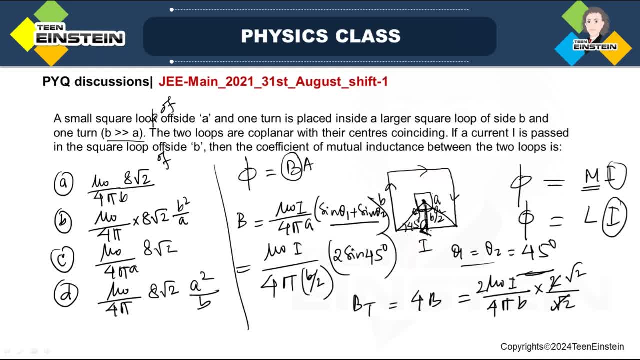 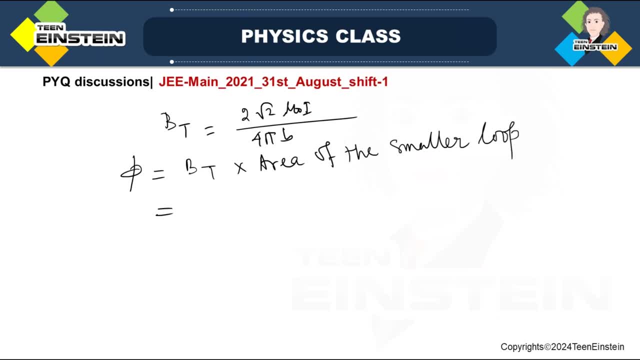 now what is the plaques fl suck will be b total into area of the area of the smaller loop. um, so smaller loop has area how much a into a area? So it will be a square. Okay, That will be a square. So 2 root 2 minus 0. I divided by: 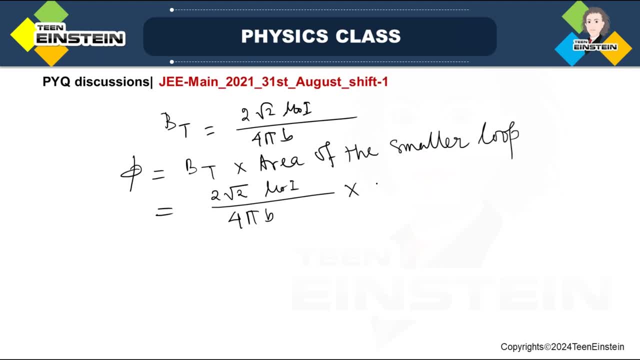 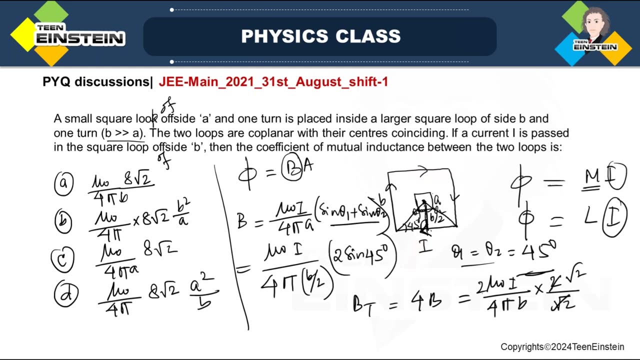 4 pi B into a square. Let us see what we have got See here. what are the options given? Okay, A square only. we have in the last option, and this might be correct, except this particular factor. We have to check. 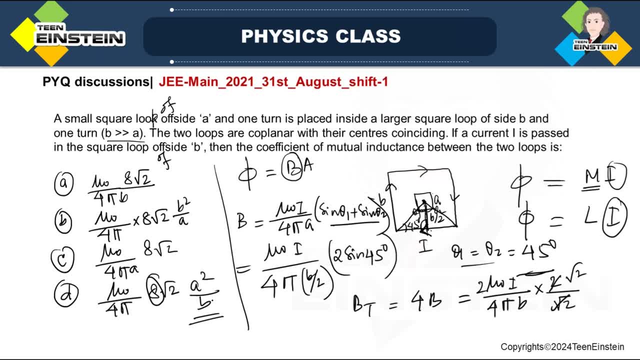 Here we have done a little mistake, maybe into 4.. Did I write No, I haven't written this 4.. Yes, So this 4 will come here. Okay, So B total, there will be 4.. So this will be. 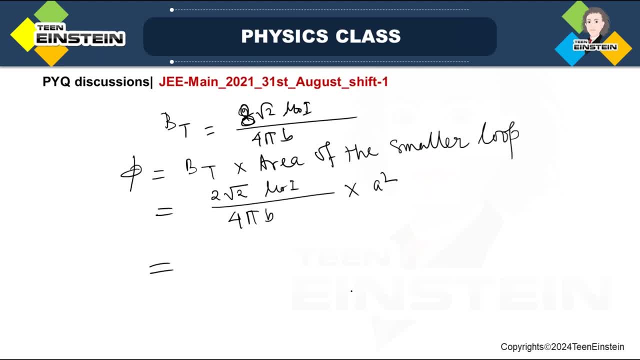 actually 8.. 8 into this. Rest of the things are all right. So this will be 8 square root of 2 divided by 4. pi B minus 0 into- I Okay, Into a square. So what we get M will be pi. 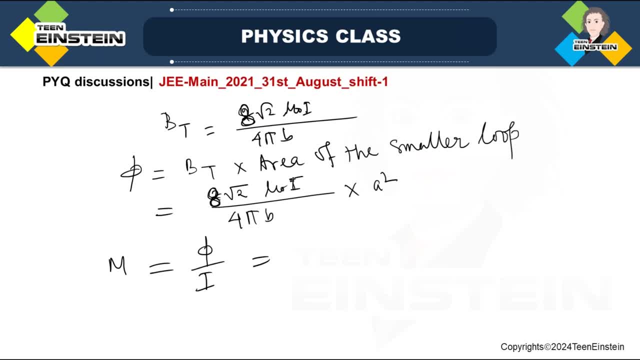 by. I So divide this, I Okay. So I have got 8 root over 2 minus 0 a square divided by 4 pi B. So in terms of: Okay. So this has got nice arrangement of this. factors: Okay, Let me write minus 0 by. 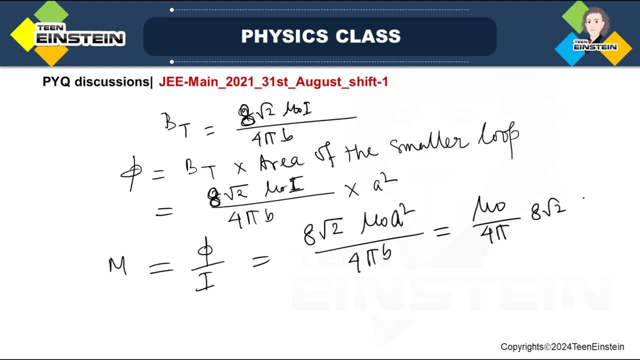 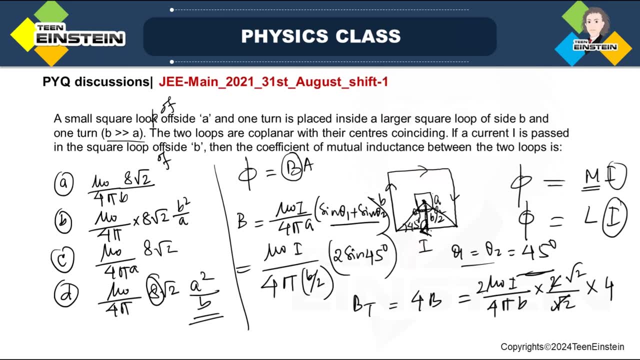 4 pi, Then 8 root over 2 and a square by B. Okay, Look this fourth option. So this is actually correct answer for this question. Okay, All right, So we have got the answer for this. D will be the correct answer. So here the bottom point is that for whatever geometry, 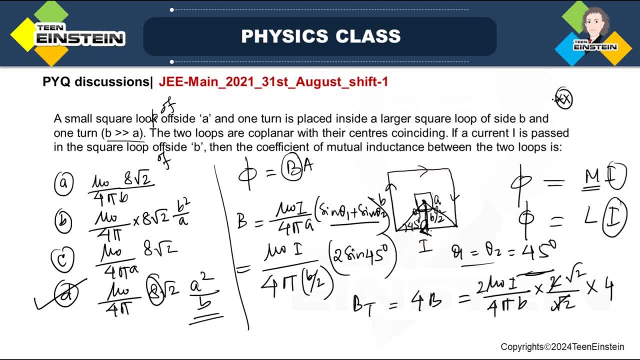 or whatever loop it may be. if you want to find out what is the mutual inductance or self-inductance, you have to find out the flux linked to that, Okay, Flux linked to that. And then, once you get the flux, you have to divide that flux with the current. 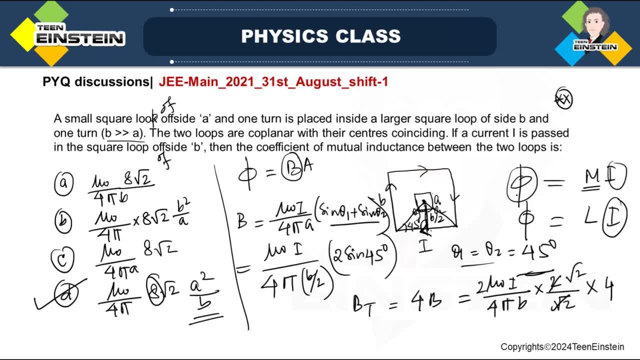 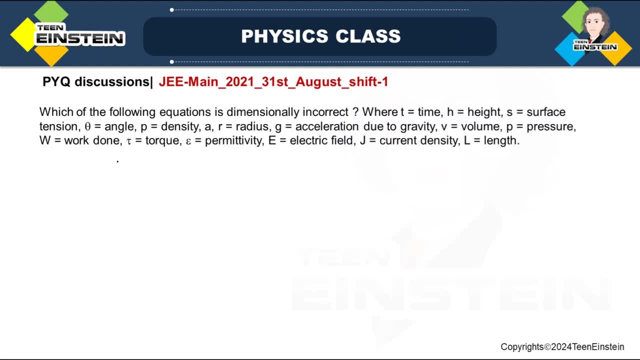 Okay, That will give you the answer. Okay, So let us now. let us solve this problem. This problem is also going to be a very interesting problem. This is from dimensional analysis. So the question- Okay Question- says: which of the following equations is dimensionally incorrect, Where T is the? 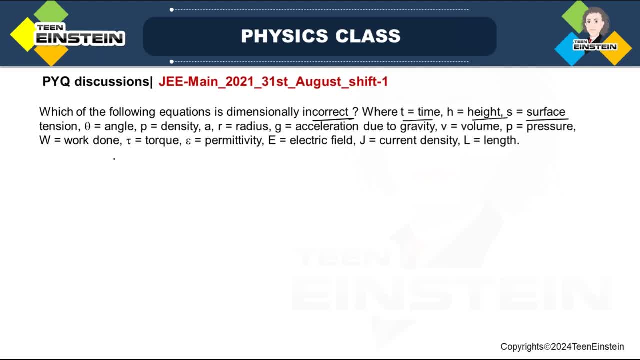 time. H is the height, S is the surface tension, theta is the angle, P is the density. Sorry, This will be rho. Rho is the density and R is the radius. Z is the acceleration due to gravity, V is the volume, P is the pressure, W is the work done, Tau is the torque. This 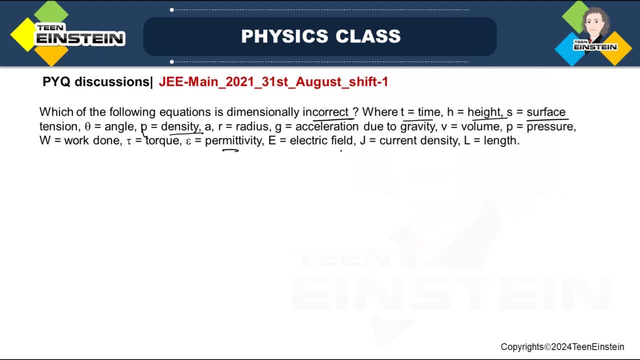 is permittivity, And E is the electric field, And J is the current density, L is the length, And let me give you the equations here. So what are the equations given? So W is equal to tau theta. Okay, First one Second. 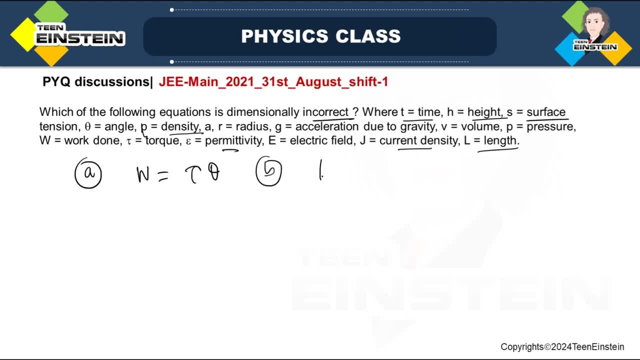 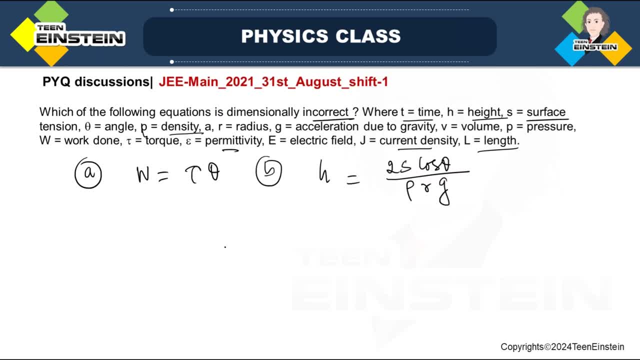 row R and G. okay, then option C, V is equal to pi. I think this is P given here. okay, let me. I think it is the row over here, row it is per 4 divided by 8. ETA L- and often D is J- is equal to del E by del T. 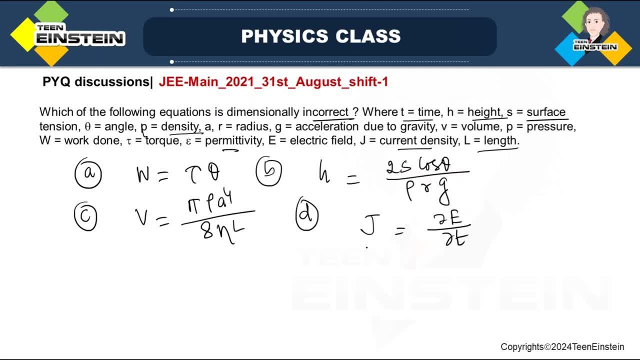 okay, we have to find out the on such course, like we have to find out the incorrect option here in terms of dimensionality. you have to check. see, this is tau. tau is the counterpart of, not counterpart. it is the. what is that called? force equivalent in the rotational mechanics? so what done in case of translational 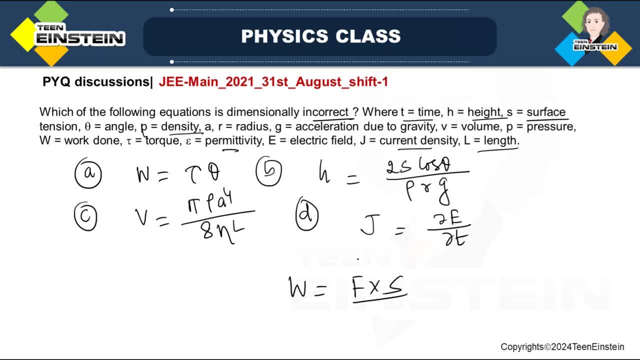 motion force in to displacement right. so here, theta is the angular displacement and tau is the fourth equivalent in the angular motion. so this is actually what- and this is true. see this expression. this is actually capillary rise, if you remember. this is: H is equal to S cost of an ORG. this is also alright capillary right. so 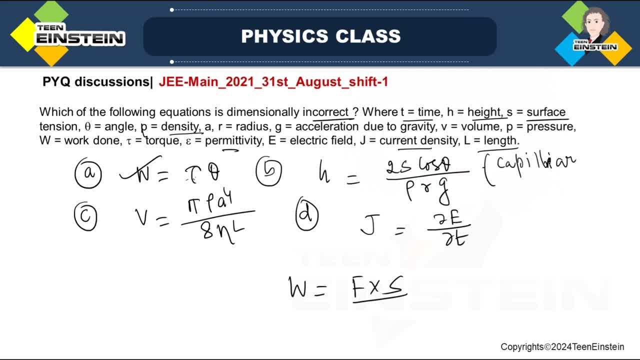 if you want to do something like this, you can do that. what you want to do is I will actually show you a little bit more ages here in this part of the video. so we are just going to do this, and also we will use a little bit of the same as before. so this: 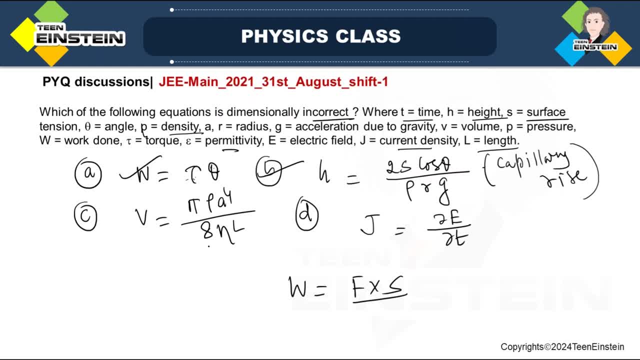 is the value of the sum of S here, this is the value of the sum of I, and this will be 1.5 S, and then the number of sources for which I will be using in some way is high. so this very cheap. I will call this capitalization right, so to say, leading to. 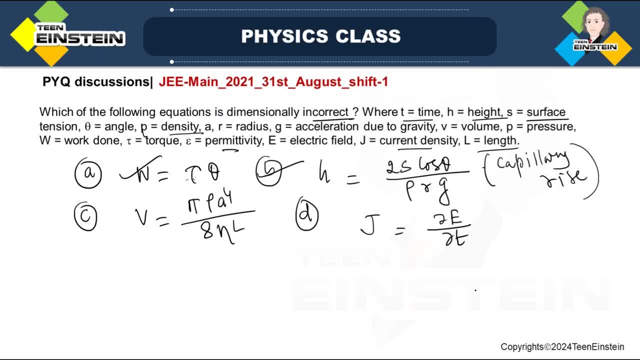 is this said right? current density means current by area. current by area, that means you know this. current by area is the current density, okay, so current has got. see. current has got unique. how much? or dimension. let us write that he by I. with that, I can write if I want to write. okay, or I. 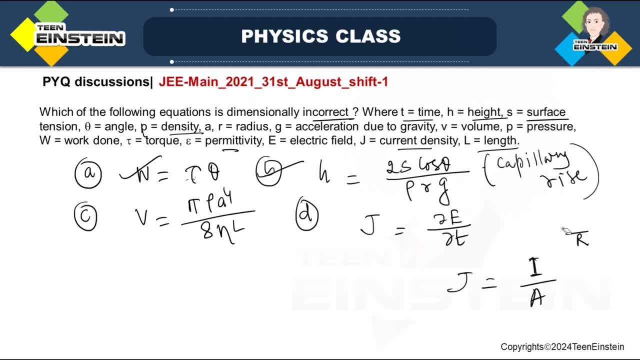 can write this: I as Q by T, Q by T. okay, so I can write Q by T. parent has got in it actually ampere. ampere by meter square. okay, ampere per meter square, but what is this unit? this is volt or this electric field is. 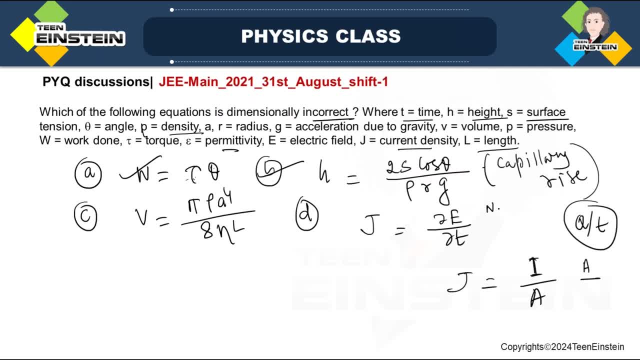 actually has got unit newton, see a physical to you. E right, it's good. oh so Newton per Coulomb, Newton per Coulomb, and this is T, so Newton per Coulomb. force: unit of force divided by charge into time. force: if force unit of force is a nuot, 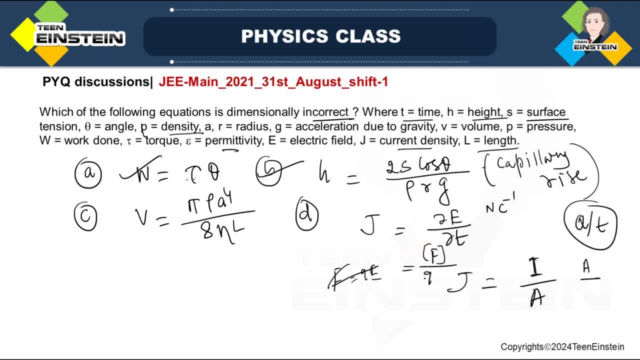 Divided by charge into time. In case of this current density, actually we don't get force and all Current divided by area. It seems to be wrong. This seems wrong. Let me confirm you. What is this. I think there was one more thing here. That's why I am. There was Epsilon over here. 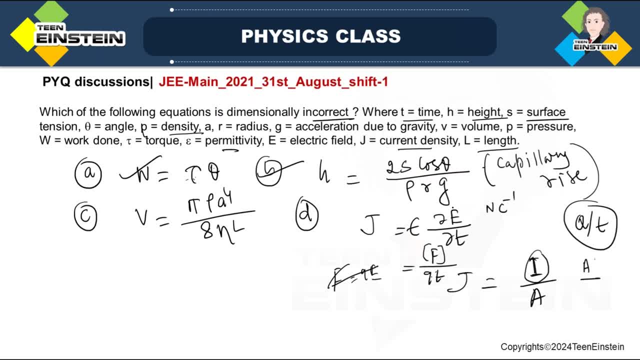 Then it is correct. Epsilon, Yes, So this will give you the density. So this is current density. This is for CO, So this is for current density. We know this is for current density. Okay, This is fine. Now it is all right, Epsilon, not into. 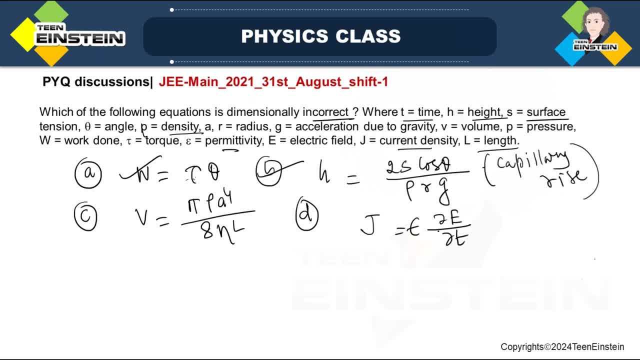 Okay, So We know electric flux, Electric flux by time, into Epsilon- Epsilon not, or Epsilon, whatever this is. This gives you displacement current. Okay, When you multiply this, pi is equal to E into A and divide that: